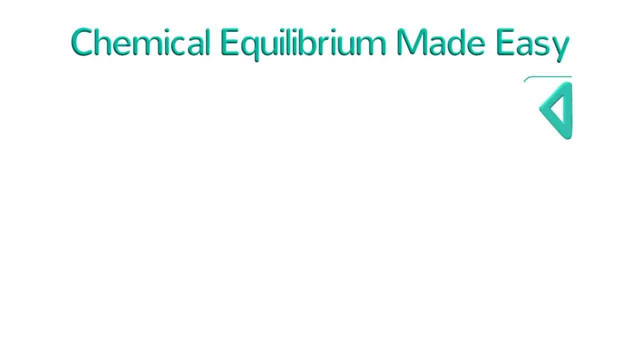 Welcome to Chemical Equilibrium Made Easy, brought to you by Ketzbook. Thank you so much to all my subscribers out there, and if you'd like to support this channel, consider becoming a patron or check out my new merch below. In this video, we're going to learn what a 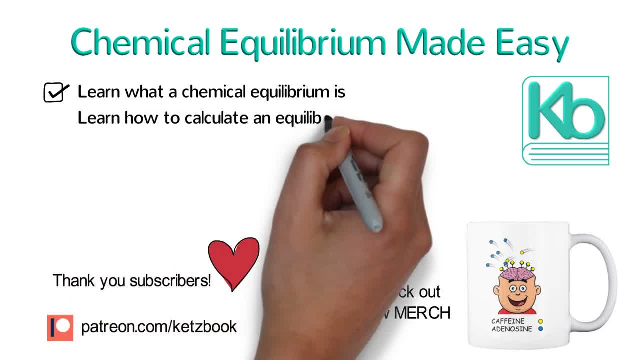 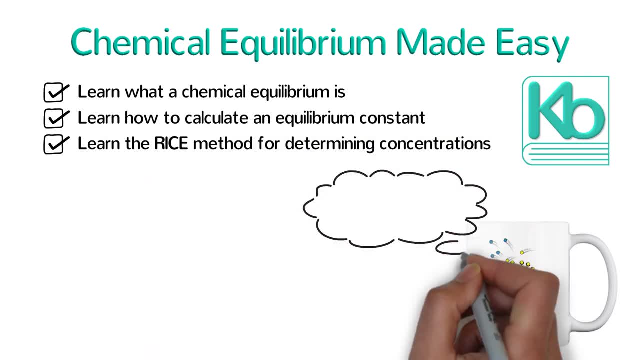 chemical equilibrium is. learn how to calculate an equilibrium constant and learn the Rice method for determining the concentration of chemicals at equilibrium. Let's start from the beginning. What is equilibrium? Equilibrium occurs when opposing forces or actions are balanced. It's kind of like a tug-of-war when the two sides pull equally. 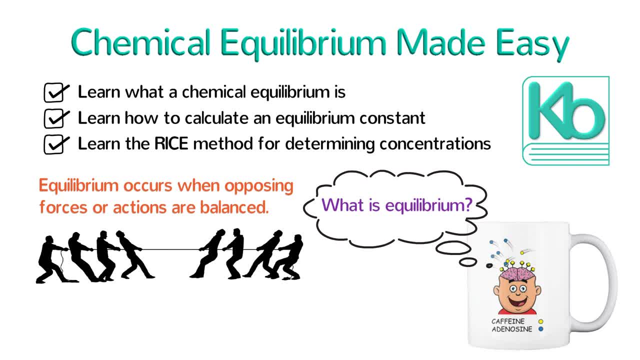 Nobody goes anywhere, even though they are pulling with a lot of force. But tug-of-war is a static equilibrium. A chemical equilibrium is a dynamic equilibrium. That is, a chemical equilibrium involves constant motion, kind of like a water fountain: The water is constantly. 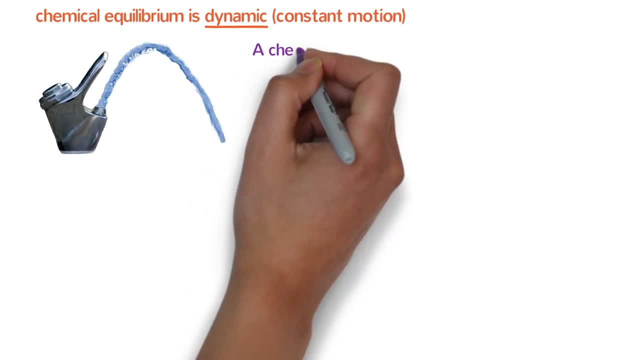 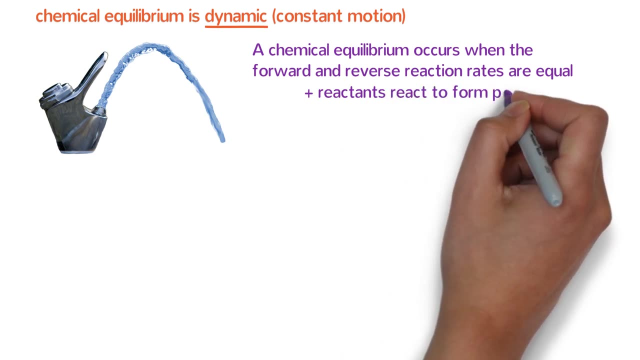 in motion, but it stays in the same place more or less. A chemical equilibrium occurs when the forward and reverse reaction rates are equal. That is, reactants constantly react to form product and products constantly react to form reactant, and the two things happen with the same speed, so that the amount of each chemical 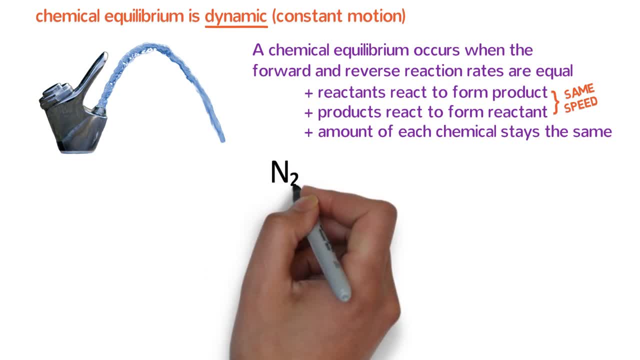 stays the same. Consider the following reaction: Nitrogen reacts with hydrogen to form ammonia. This reaction is known as the Haber-Bosch process and like nearly all reactions, it can also go in reverse. That is, ammonia will also decompose to reform. 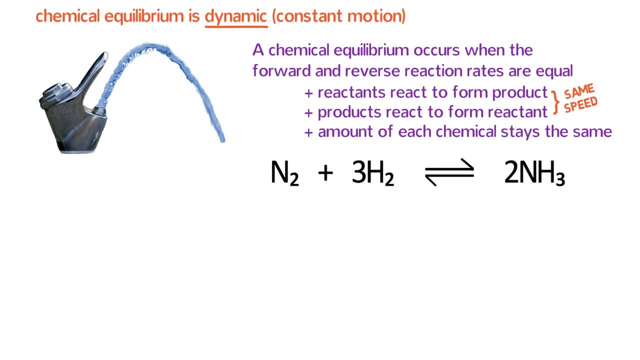 nitrogen and hydrogen. does that look like? Suppose that we have a 1 liter container and we fill it with 2.8 moles of nitrogen, 4.4 moles of hydrogen and an appropriate catalyst. We heat the mixture to 450 degrees. 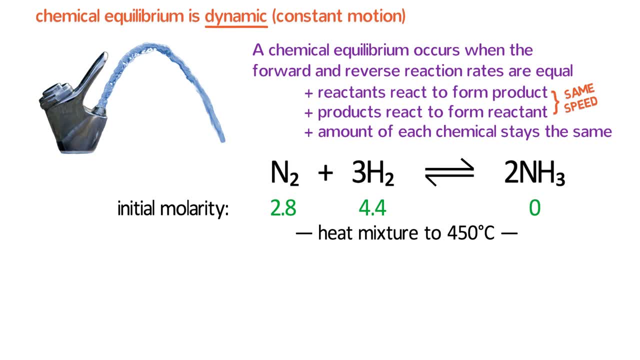 Celsius and we observe that the concentration of nitrogen and hydrogen decrease as they turn into ammonia. After a while, however, the concentrations of nitrogen, hydrogen and ammonia no longer change. There are 2 moles of nitrogen, 2 moles of hydrogen and 1.6 moles of ammonia. Those amounts 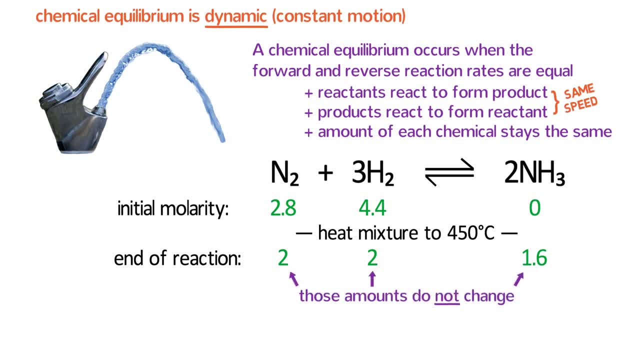 do not change, no matter how long you wait. You might think that the reaction has stopped, but it hasn't. Rather, the reaction has reached equilibrium, That is, the chemicals are still reacting and never stop reacting. The amounts do not change because new ammonia is formed at the 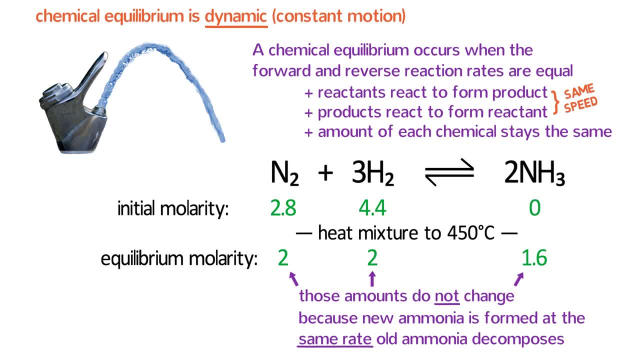 same rate old ammonia decomposes. Keep in mind that equilibrium is not a special type of reaction. In fact, nearly all chemical reactions are equilibrium reactions. They just might not appear that way. Now we can use our knowledge of kinetics to describe an equilibrium in a very useful way. 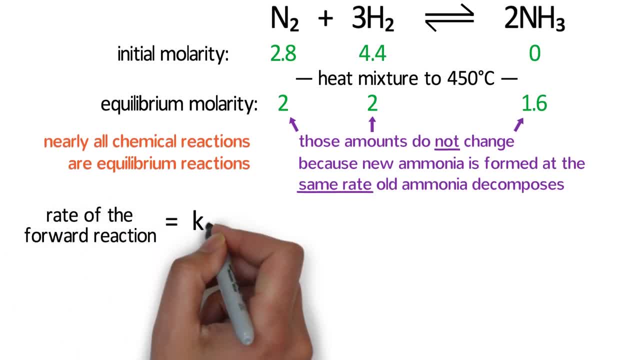 For the Haber process, the rate of the forward reaction is a rate, constant times the molarity of nitrogen times the molarity of hydrogen raised to the third power. Remember that a rate law is typically just a constant times the reactants raised to the power of their coefficients. 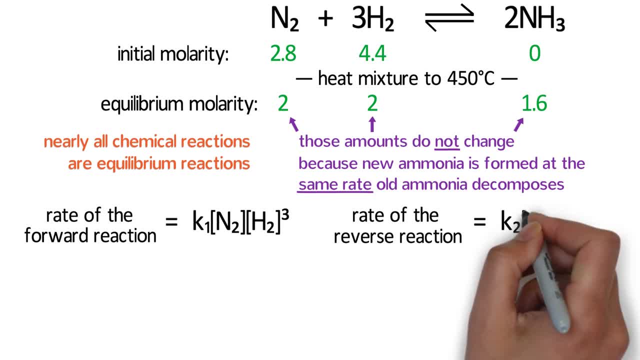 Likewise, the rate of the reverse reaction is the rate of the forward reaction times. the rate of the reaction raised to the power of the reaction. The rate of the reaction is the rate of the reaction raised to the power of the reaction. The reaction is the rate of the reaction. The. 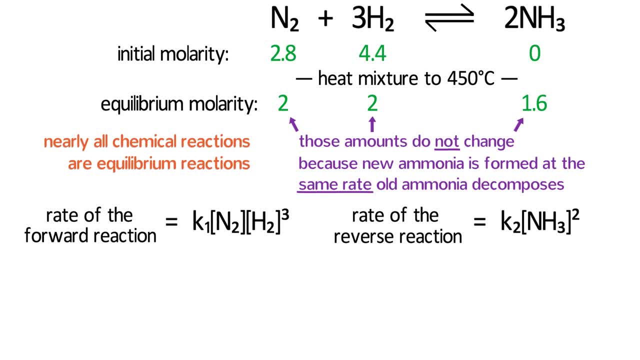 reaction is the rate of the reaction. The reaction is the rate of the reaction. Remember that at equilibrium, the forward and reverse reactions occur at the same rate, so these two expressions are equal. I'm going to erase the words so that we can focus on the two equal rate laws. 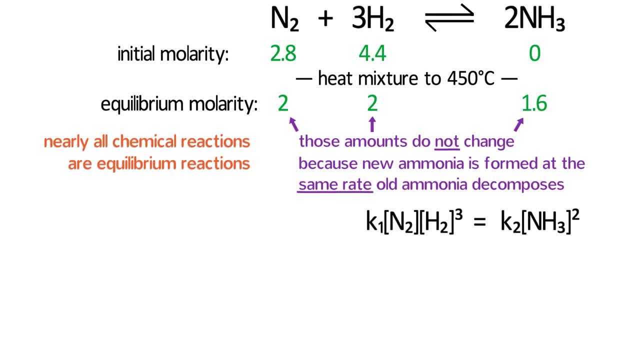 Now what I want to do is to put all the variables on one side and the constants on the other. so let's see what happens if I divide both sides of the equation by K2, N2, H2 to the third. On the left side, N2 over N2 cancels out, as does H2.. 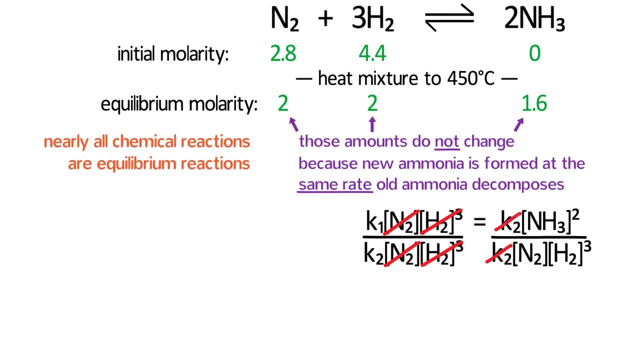 H2 over H2.. On the right side, K2 over K2 cancels out. That leaves me with K1 over K2. equals NH3 to the second over N2H2 to the third. Because K1 and K2 are both constants, their ratio is also a. 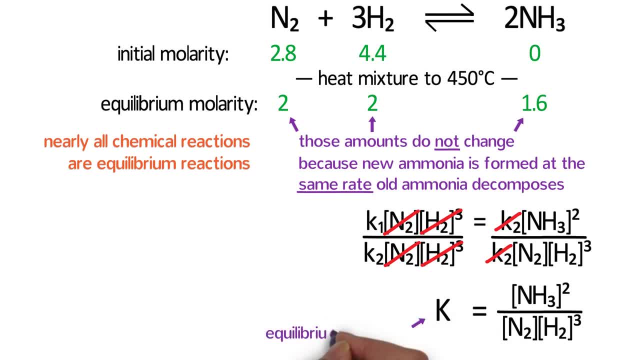 constant and that is a special constant that we call the equilibrium constant. We call this constant KEQ for equilibrium constant, or KC for the concentration equilibrium constant, or simply just K, capital, K, that is, Lowercase k is for rate constants and uppercase k is for equilibrium. 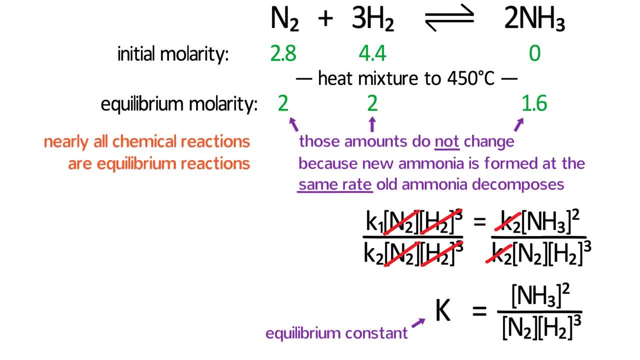 constants. The equilibrium constant is a physical constant for a specific reaction at a specific temperature and it tells you about the reaction In general. the equilibrium expression of any reaction is that the equilibrium constant is equal to the molarity of the products raised to the 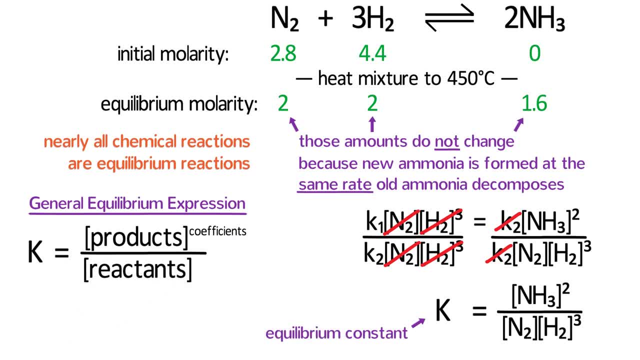 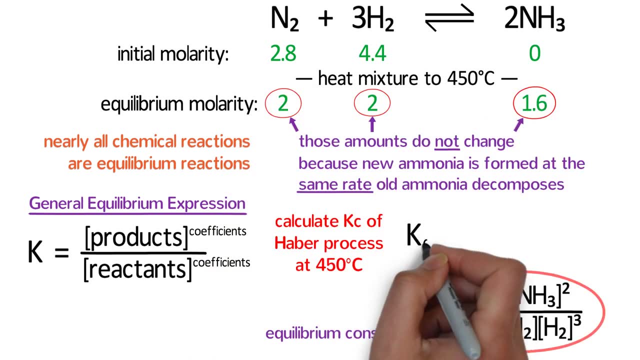 power of their coefficients divided by the molarity of the reactants raised to the power of their coefficients. Let's calculate the equilibrium constant of the Haber process at 450 degrees Celsius. To do that, we are going to use the equilibrium expression of the Haber process and plug in the molarity at equilibrium. KC equals 1.6. 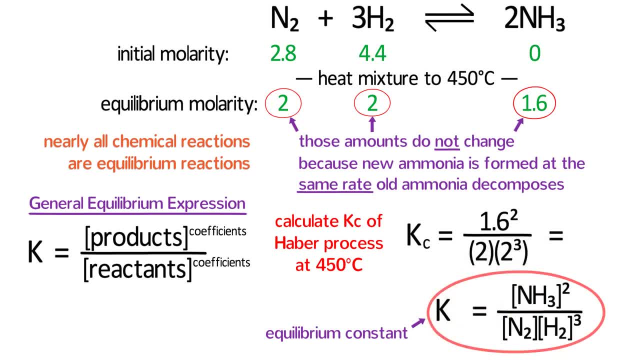 squared divided by 2 times 2 cubed, which equals 0.16.. Interestingly enough, equilibrium constants are unitless because the concentration values we use in the calculation are all relative to the standard concentration, that is, relative to 1 mole per liter. But what is the equilibrium? 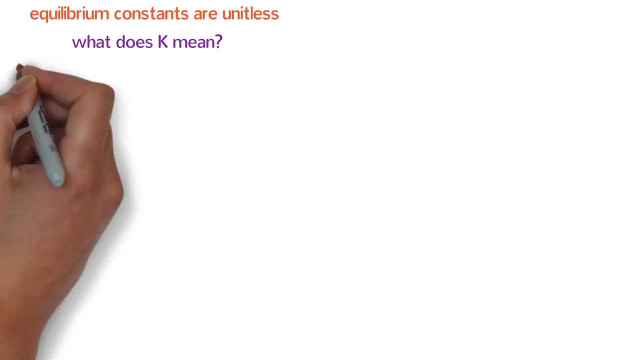 constant even mean. A large equilibrium constant, that is, if K is greater than 1, means that the reaction is product favored. It will tend to make more products than reactants. A small equilibrium constant, that is, if K is less than 1, means that the reaction is reactant favored and it will tend 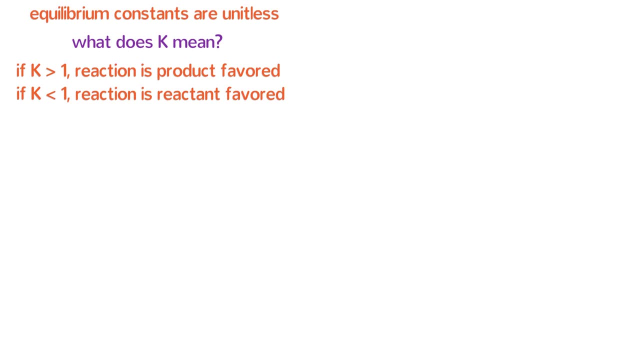 to make less products than reactants. Let's consider another reaction. Carbon tetrachloride decomposes at 700 Kelvin to make elemental carbon and chlorine gas. The concentration equilibrium of that reaction should be equal to the molarity of the products raised to the power of their. 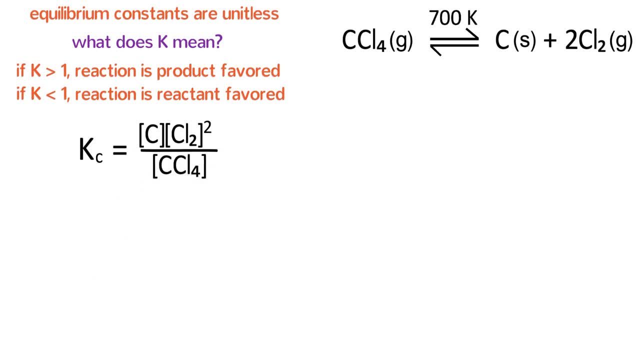 coefficients divided by the molarity of the reactant raised to the power of its coefficient. However, carbon is a solid, so what is its molarity? The molarity, or, more correctly, activity, of any solid or non-homogeneous reactant or product has a value of 1.. That means that we 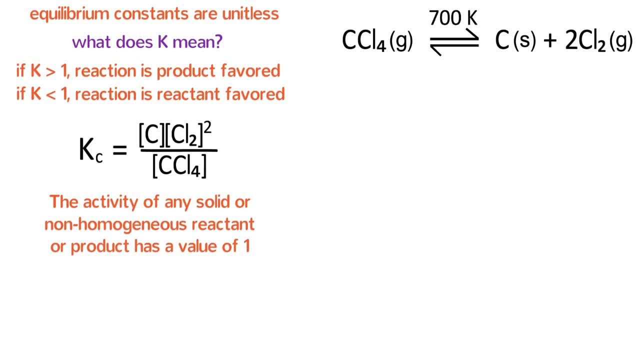 can exclude all solids or non-homogeneous chemicals from the equilibrium expression, so the molarity of carbon should be erased. In addition, solvents typically have an activity of 1 and are not written in the equilibrium expression. Let's try another problem. Suppose that 1 mole of carbon tetrachloride is added to a 5-liter flask. 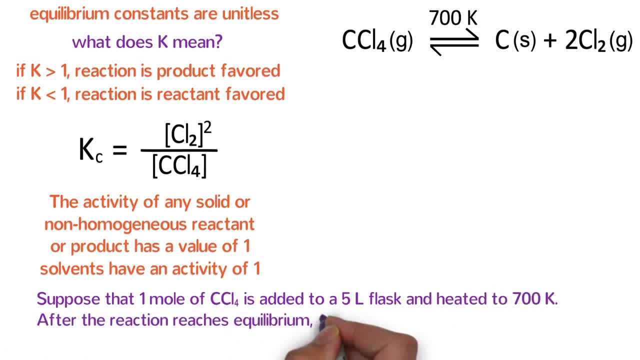 and heated to 700 Kelvin. After the reaction reaches equilibrium, there are 0.88 moles of carbon tetrachloride remaining. Calculate the equilibrium constant of the reaction. When faced with a problem like this, the best way to solve it is to set up a rice chart. 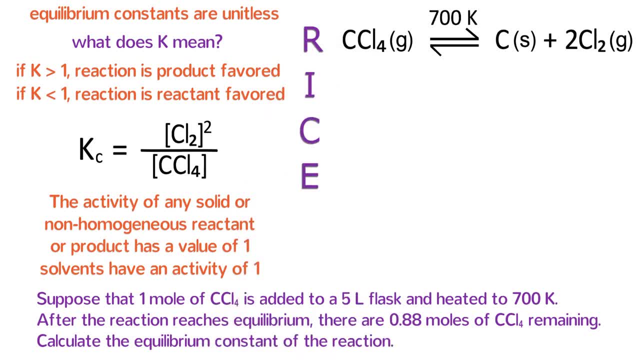 That's right, R-I-C-E. Whenever you solve an equilibrium problem, the R stands for reaction and we already have our balanced reaction written. The I stands for initial molarity, the C stands for change in molarity and the E stands for equilibrium. 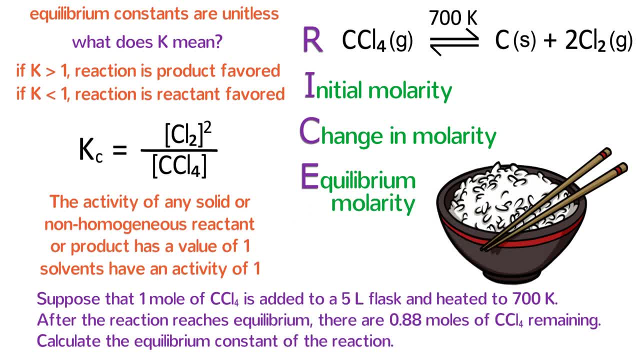 molarity. Be sure to actually write out R-I-C-E so that you don't skip anything or make a mistake. The question tells us that we are starting out with an initial amount of 1 mole of carbon tetrachloride in a 5-liter flask, so we can calculate its initial molarity using the equation. M equals N over V, which is 1 mole of carbon tetrachloride. So we can calculate its initial molarity using the equation M equals N over V. and we can calculate its initial molarity using the equation M equals N over V. 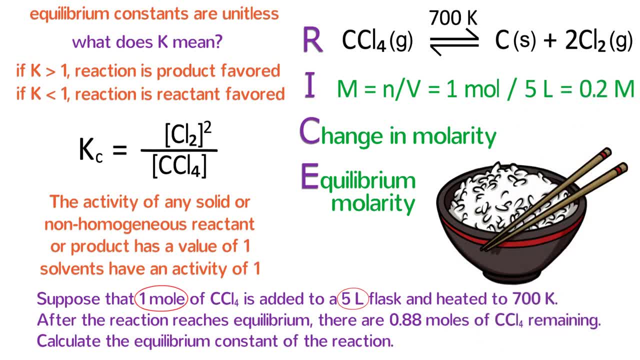 which is 1 mole divided by 5 liters, or 0.2 molar. We put the 0.2 directly under the CCl4.. We can ignore carbon because it is a solid and there is initially no chlorine gas. 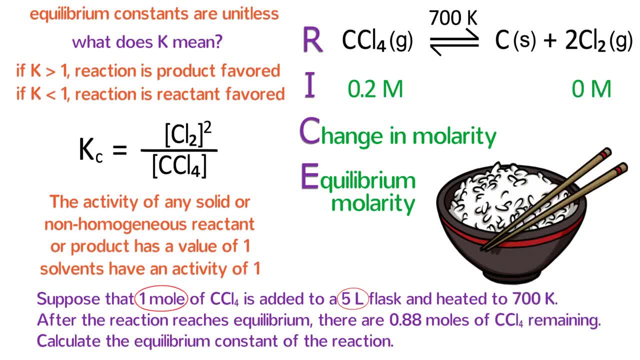 so we put a 0 underneath Cl2.. As for the change in molarity, we know that the reactants are decreasing by a certain amount. so we put minus X for CCl4, and the coefficients tell us that 2 Cl2 are made for every 1 CCl4 that is lost. so we put plus 2X for Cl2.. 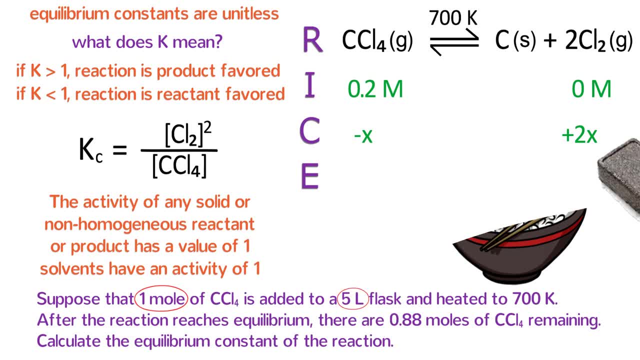 The equilibrium molarity is simply the initial molarity plus the change in molarity. so that is 0.2 minus X for carbon tetrachloride and 2X for chlorine. Now how do we figure out X? Looking back at the problem, it says that there are 0.88 moles of 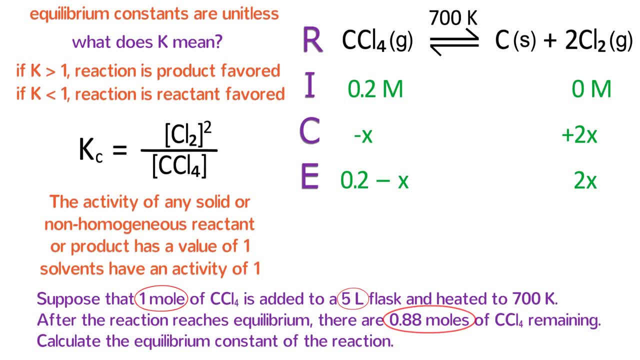 CCl4 at equilibrium. so we can calculate the equilibrium concentration of carbon tetrachloride, which is 0.88 moles divided by 5 liters, or 0.176 molar. The equilibrium molarity of CCl4 is also equal to 0.2 minus X. 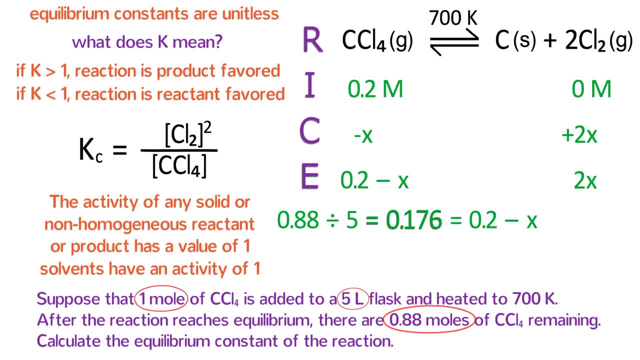 If we add X to both sides and subtract 0.176 from both sides, we can calculate X to be 0.2 minus 0.176, which equals 0.024.. Now the only thing left is to plug in the. 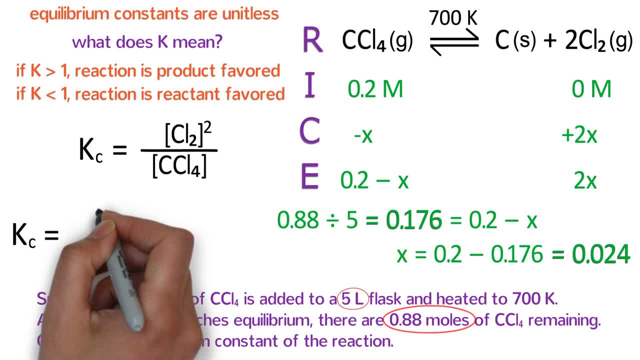 numbers and calculate the equilibrium constant. Kc equals the equilibrium molarity of chlorine squared divided by the equilibrium molarity of carbon tetrachloride. The equilibrium molarity of chlorine is 2X, and we can substitute 0.024 in for X. 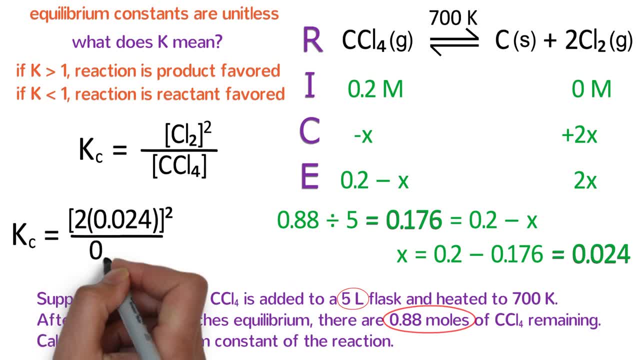 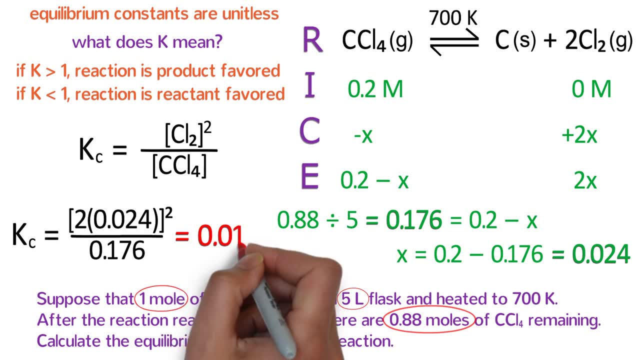 We already calculated the equilibrium molarity of CCl4 to be 0.176.. Plugging this into our calculator gives us an equilibrium constant of 0.013.. Does this number make sense? Yes, the concentration of reactants is larger than the concentration. 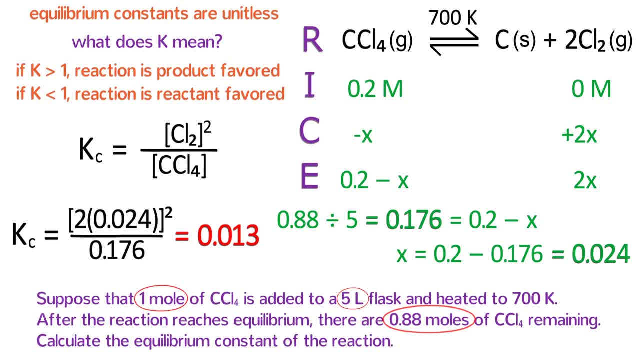 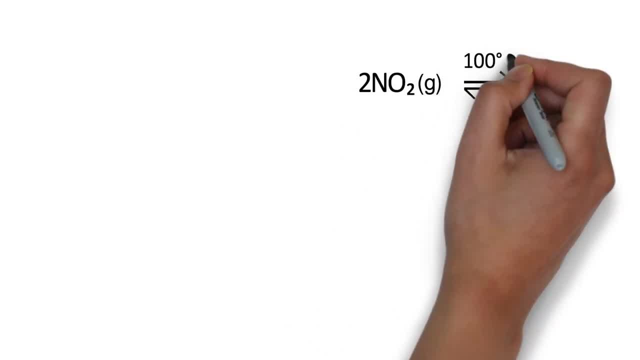 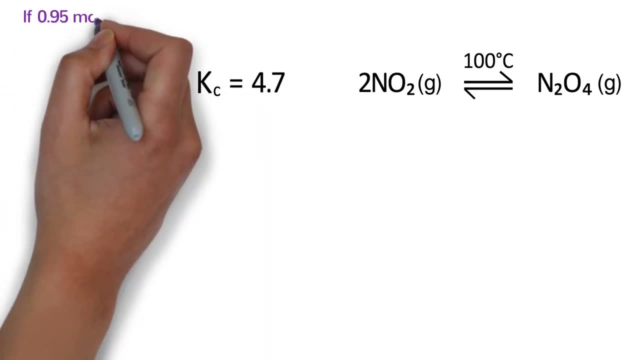 of products at equilibrium. so an equilibrium constant less than 1 makes sense. Okay, let's try one more equilibrium constant. In our equilibrium problem nitrogen dioxide dimerizes at 100°C to make dinitrogen tetroxide. Under these conditions, Kc equals 4.7.. If 0.95 moles of dinitrogen tetroxide is added, 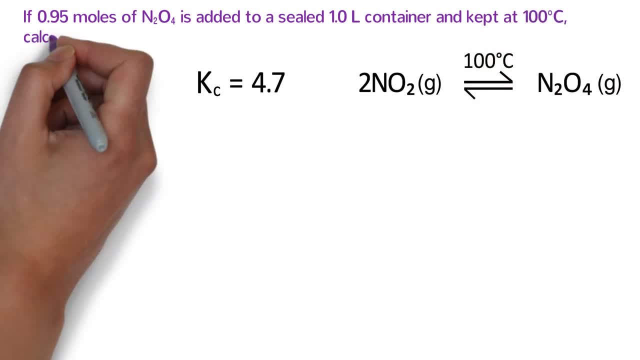 to a sealed 1-liter container and kept at 100°C. calculate the equilibrium concentrations of nitrogen dioxide and dinitrogen tetroxide. Like most equilibrium problems, it is best to start by making a rice table. We already have the balance reaction. 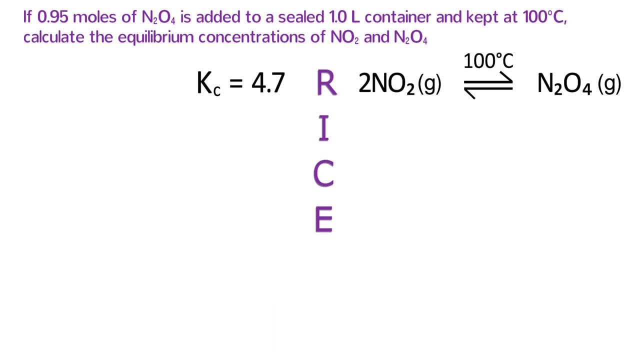 This problem states that we are starting with N2O4,, which is our product, so the initial molarity of NO2 is 0, and the initial molarity of N2O4 is 0.95.. As this reaction progresses, the amount of nitrogen dioxide should increase, so the change. 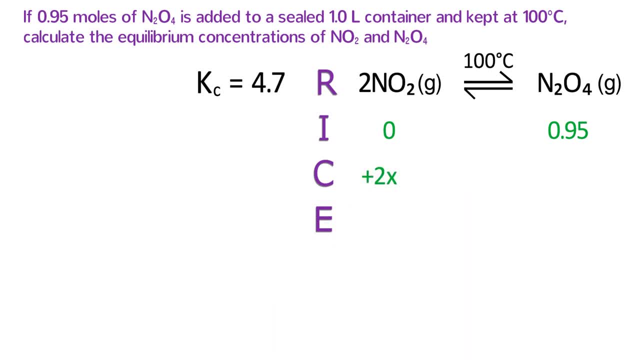 in NO2 should be plus 2X. The 2 comes from the coefficient in the balance reaction. Because the reaction will progress to the left, the N2O4 molarity will decrease, so its change should be minus X. To get the equilibrium molarity, simply add the initial molarity to the balance reaction. 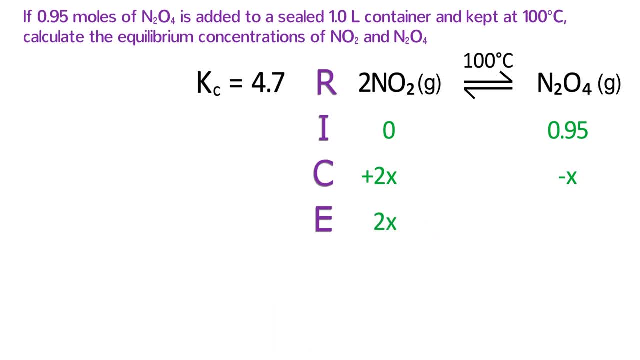 The result is 2X for NO2 and 0.95 minus X for N2O4.. Next let's write out the equilibrium expression. KC equals the molarity of N2O4 on the top, because it is the product and there is no. 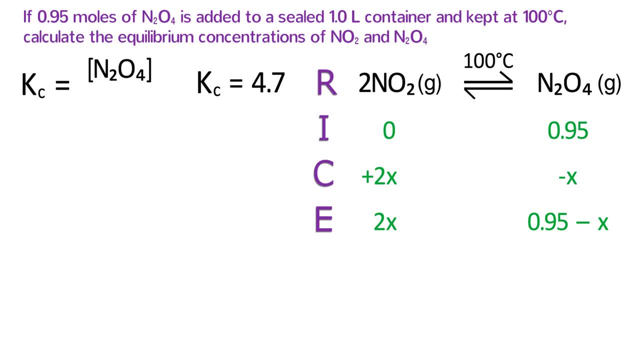 exponent, because N2O4 has no coefficient in the balance reaction, divided by the molarity of NO2, squared because NO2 has a coefficient of 2 in front of it in the balance reaction. We already know that the equilibrium constant equals 4.7.. 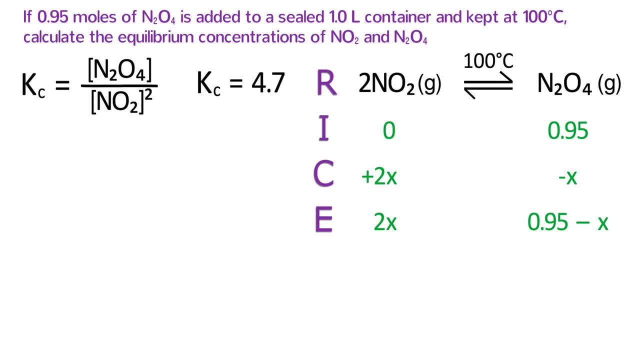 Now let's write out the equilibrium expression. Now we can plug in the equilibrium values and solve for: X Substitution gives us 0.95 minus X divided by 2X squared equals 4.7.. We can eliminate the fraction by multiplying both sides by 2X squared, which yields 0.95. 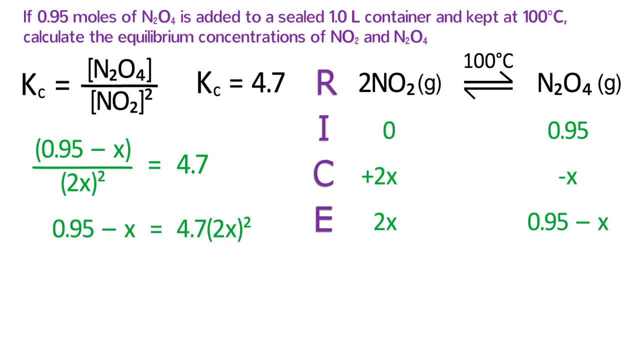 minus X equals 4.7 times 2X squared. By now we can see that this is a quadratic equation, so let's put it in a form that enables us to plug it into the quadratic formula. Subtract 0.95 and add X. 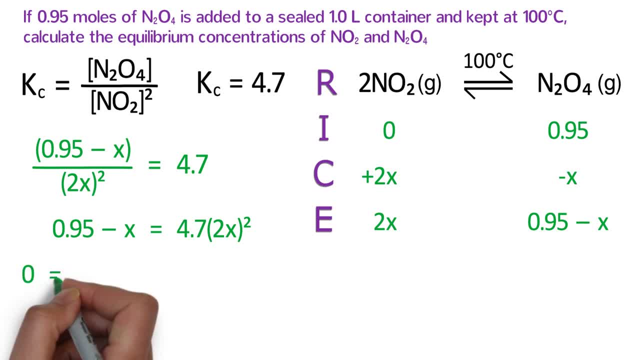 Subtract X to both sides of the equation. This gets us 0 equals 18.8X squared, plus X minus 0.95.. The 18.8 comes from 4.7 times 2 squared. Now we can plug those coefficients into the quadratic formula. 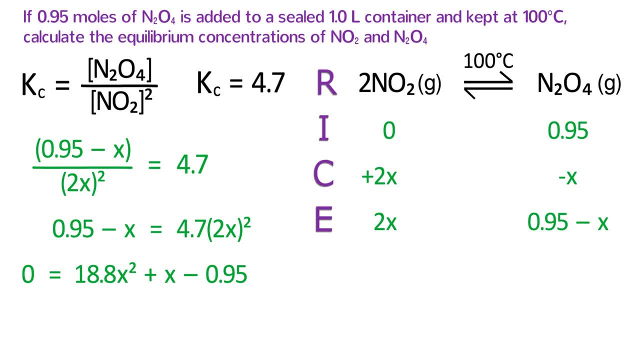 Hopefully you have a calculator that can solve this or you can program an equation into your calculator to solve it. If not, just use the quadratic formula to calculate it yourself. In this case, A is 18.8.. B is 1.7.. 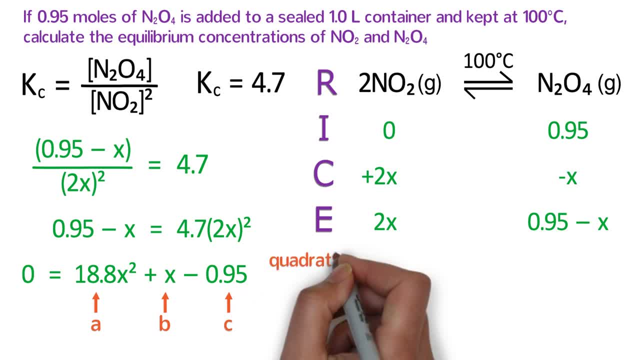 And C is negative 0.95.. The result from the quadratic formula is that X equals 0.2 or negative 0.25.. Now pause here and think about those two values. Which is the correct value for X? The negative value does not physically make sense because that would mean a negative concentration. 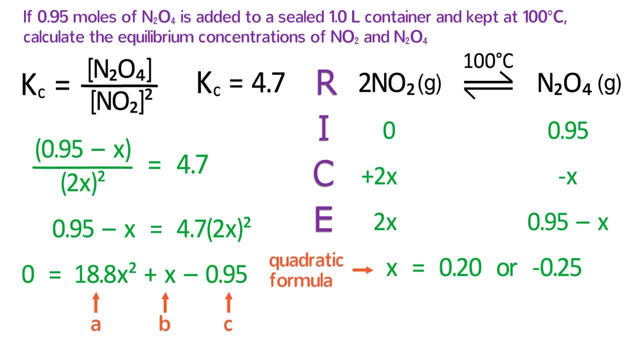 of NO2 at equilibrium, which of course is impossible. So X equals 0.2.. Last of all, we plug this value of X back into our equilibrium values. on the rice table, The nitrogen value of X equals 0.2.. 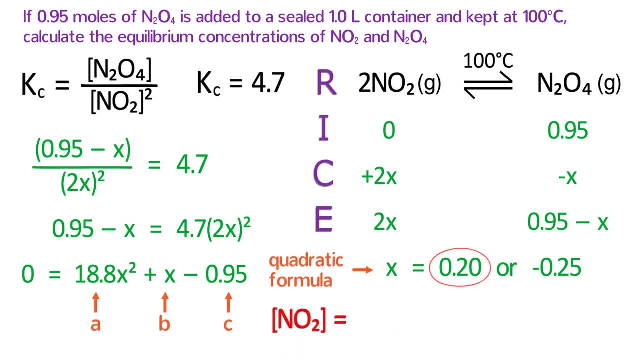 We plug this value of X back into our equilibrium values on the rice table. The nitrogen dioxide molarity is 2 times 0.2, which is 0.4 molar. The dinitrogen tetroxide molarity is 0.95 minus 0.2, or 0.75 molar.